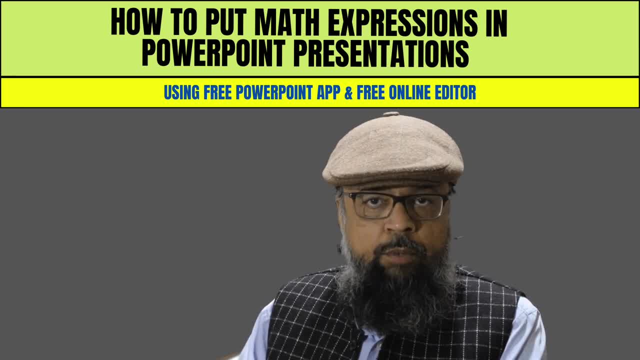 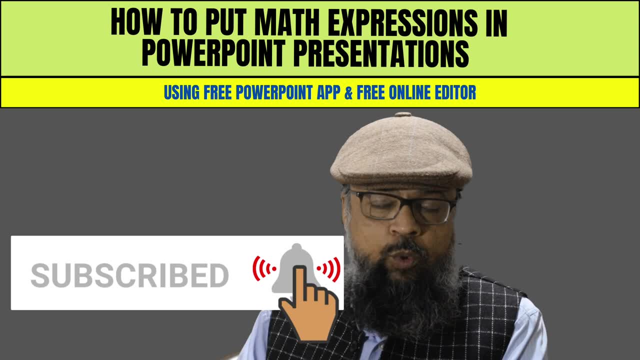 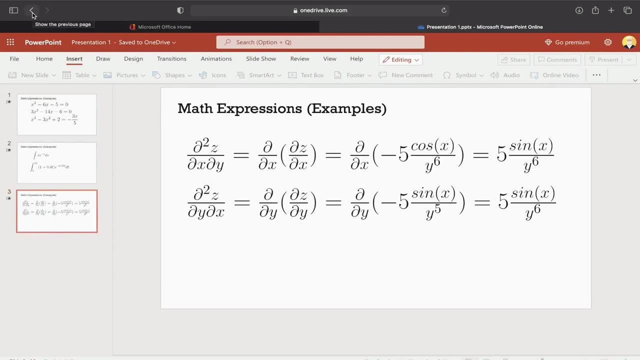 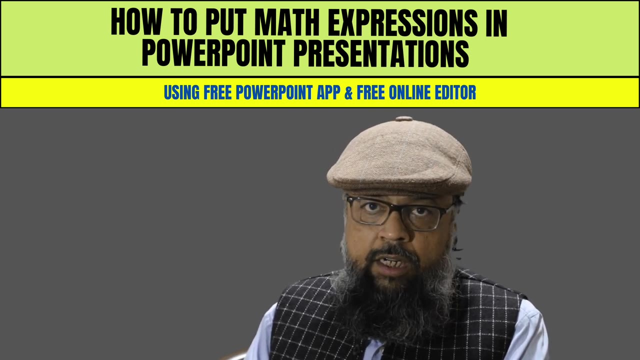 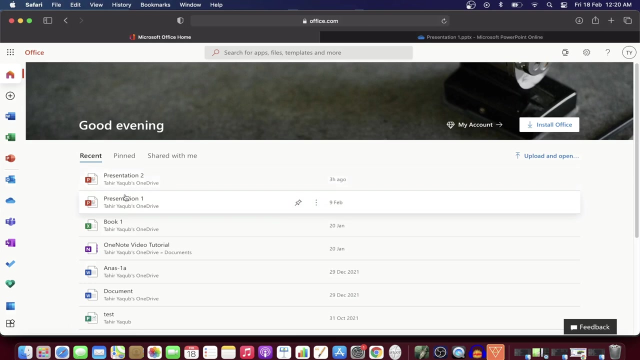 Hello and welcome to my channel. My name is Tahir. I make videos about educational technology tools. If you are interested in this topic, please hit the subscribe button and also the notification bell to get notified whenever I post a new video on this channel. Now, PowerPoint is a software of choice when creating presentations for most of us, Although I use other methods such as latech and Canva for creating my presentations, and Microsoft PowerPoint app is freely available on officemicrosoftcom website. But if you 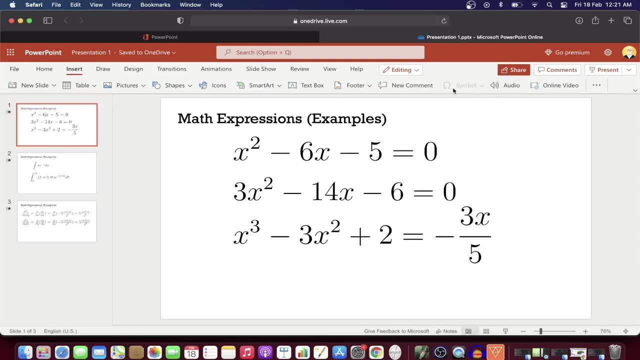 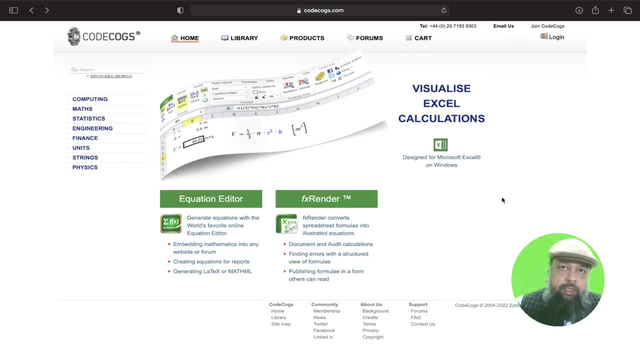 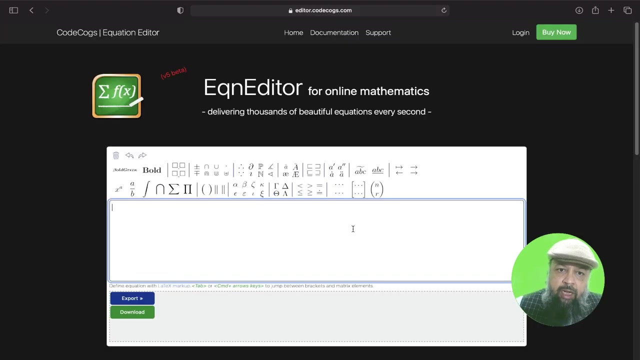 look at the insert tab, there is no equation editor available. So let us see how we can write math expressions in our PowerPoint presentation. And the equation editor which we are going to use to type math expressions and math equations is called code cogs. and simply type code cogscom in any of the browsers you are using, then click on equation editor, And this editor is a latech based editor. But don't get scared that you will have to use a latech based editor. So let's get started. 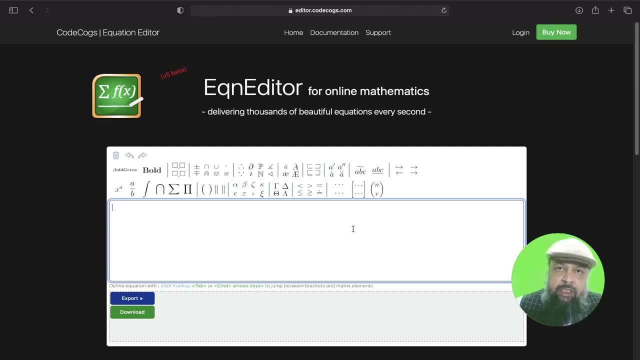 to use some programming. you only need less than 10 latech commands to understand, which I'm going to show you next. And once you understand those commands, you will be able to create most types of math expressions for your presentations or for your lectures. So let me show you how many scientific notations and symbols are available in this latech editor. So if you hover over these icons, you will see that there are few. 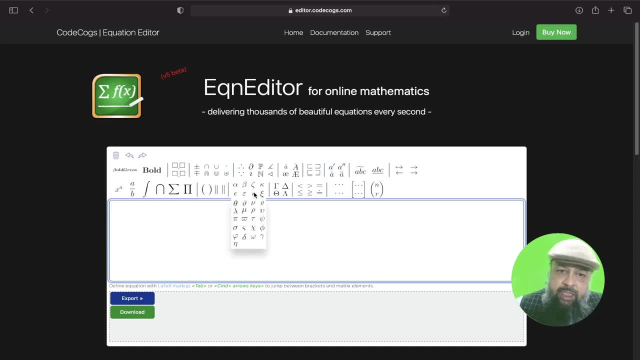 fonts available, then if you hover over these Greek symbols, for example, it will show you the symbols as well as the latech command to print those symbols. So, for example, if you type backslash zeta, the symbol zeta will be printed. Similarly, all other Greek symbols are available. all types of brackets and parentheses are available. you can type all kinds of matrices, determinants and curly brackets. you can type permutations. 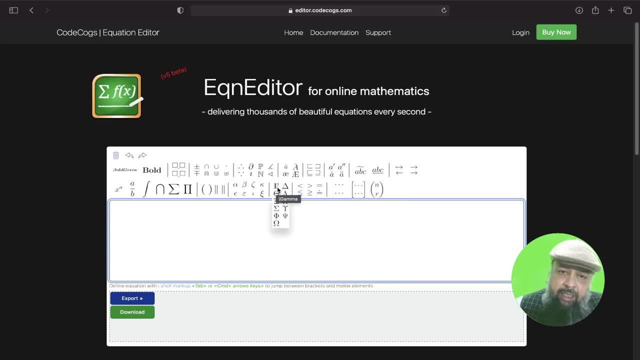 symbols here. then there are capital Greek letters Also. sometimes you have to use these types of arrows and curly braces. there are a lot of arrows available, then angle signs are available, And then also there are few stars, squares, rectangles and other shapes are available. So first I'm going to type few equations and put them in my presentation, And then I will show you those latech commands. 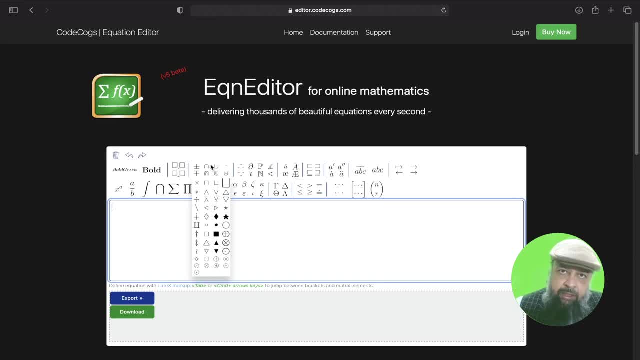 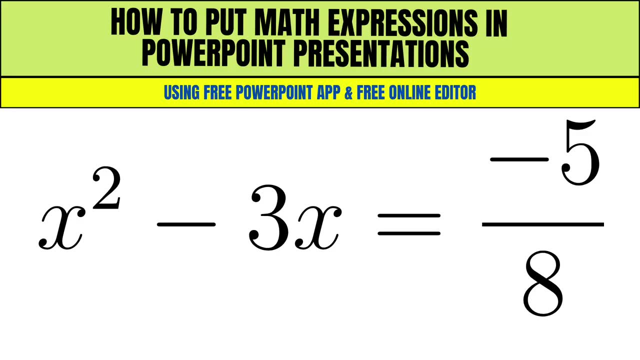 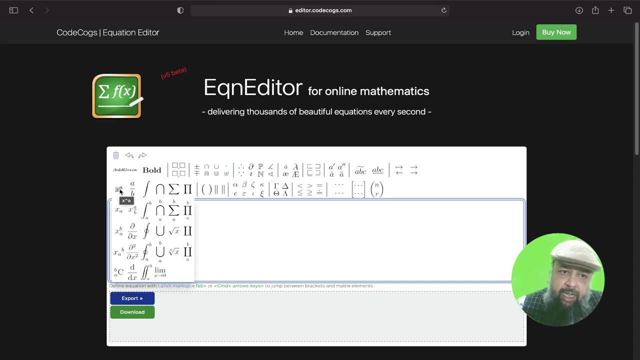 that will help you create all kinds of math equations. So let me type something. So I have this equation which you can see on the screen, and I'm going to type this. So, in order to type x square, I hover over this x raised to the power a, And it also shows me how to type x raised to the power a in latech. So you type x, then hat and then a. So this is what I'm going to do here. So x hat, which is shift. 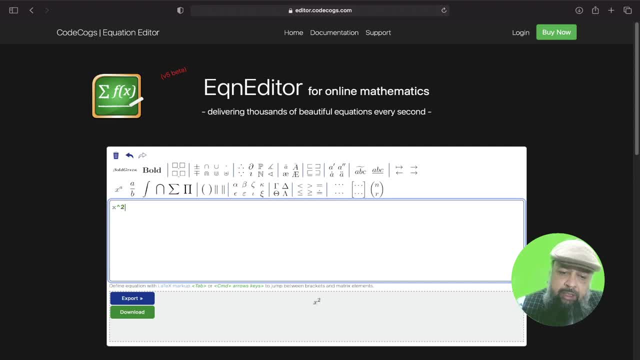 six on my keyboard and then two. then minus three x equals. and now I have to type a fraction. To do that, if I hover over this a divided by b, it shows me how to type a fraction in latex, which is backslash frac. then within curly brackets you type the numerator, which is a, and then the denominator, which is b. So if you type like this, it will type a fraction for you, So you can click on that And it 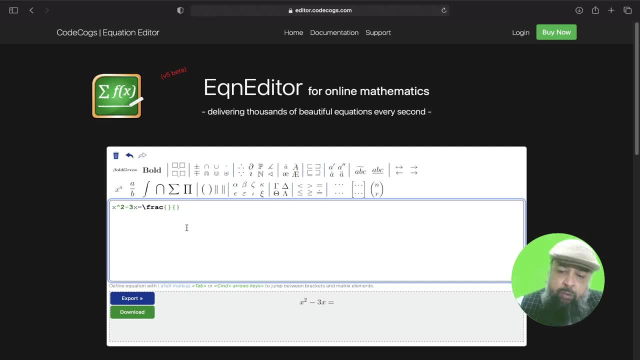 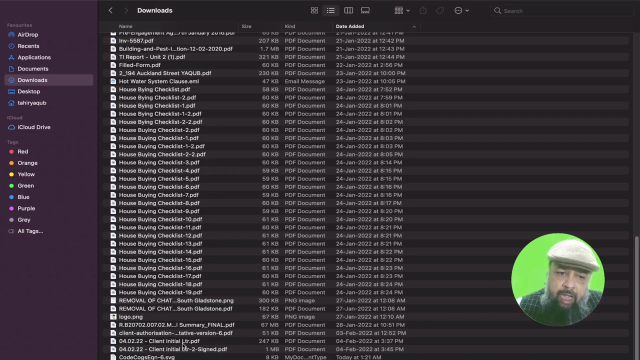 will show you where you have to type the numerator. So my numerator is minus five and my denominator is eight. And now at the bottom I can see that I have created this math equation And now my equation is ready to be downloaded. In order to download the SVG file for this math equation, I click on download And now in my download folder at the end I can see this code: cogs equation dot SVG. 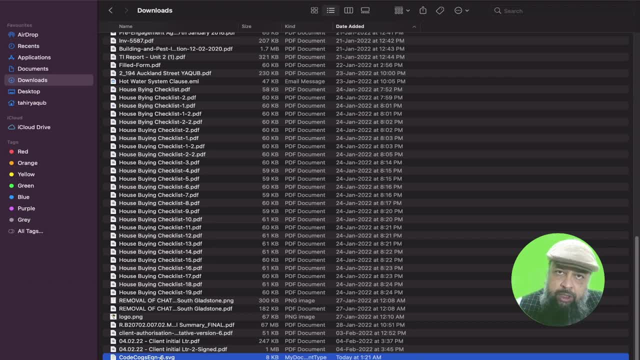 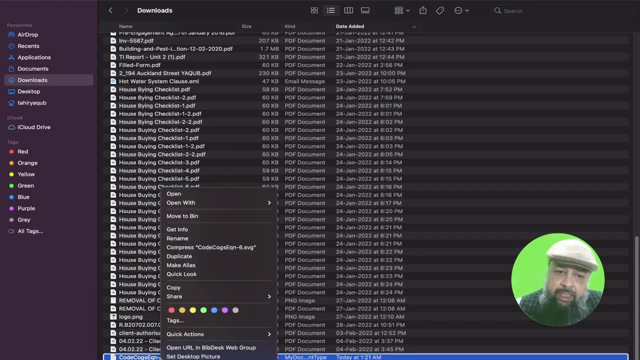 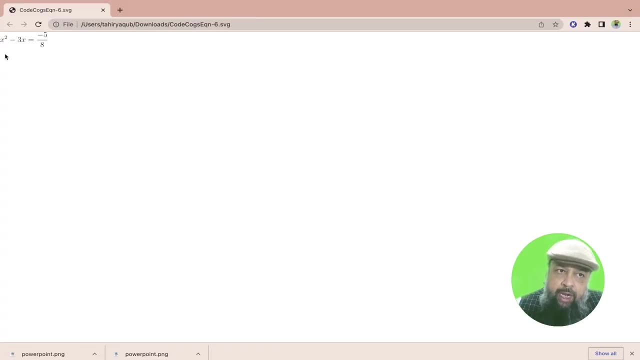 This is the default name given by the equation editor, And remember that if you want to view this file, you can view in your browser. So if I right click and I click on open with Google Chrome, it will open a new browser window and it will show me this SVG file. But I want to insert this file in my PowerPoint presentation, So let me close this And now I copy this file, dot SVG. 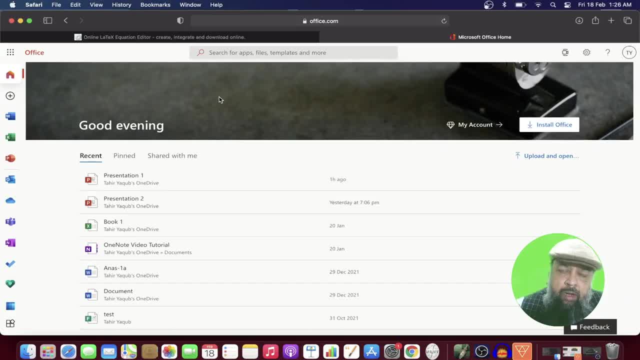 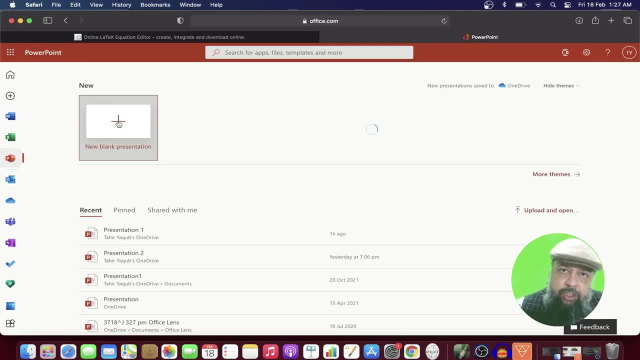 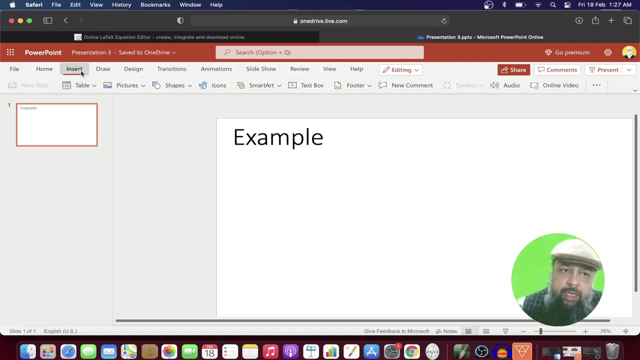 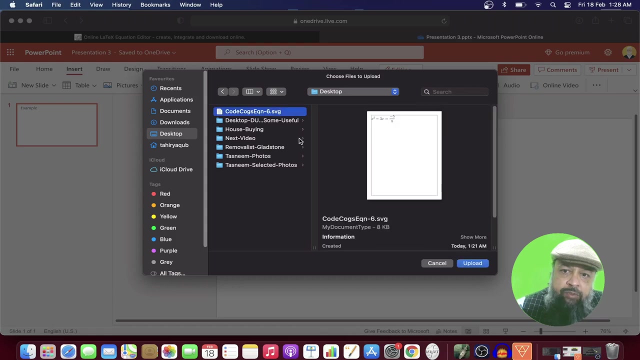 And now I paste this file on my desktop. And now I go to Microsoft Office website and click on PowerPoint. I start up blank presentation and I can give it a title if I want, And now I click on insert picture this device. and from my desktop I click on this SVG file and I click upload and on. 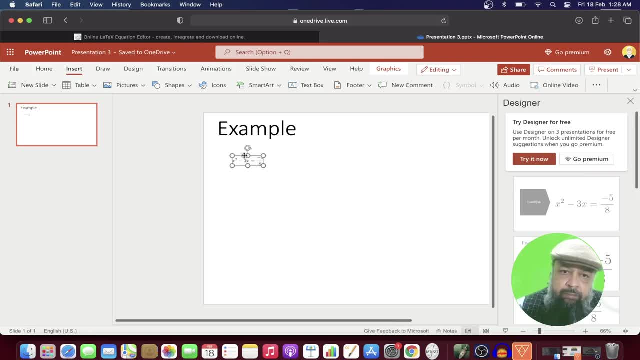 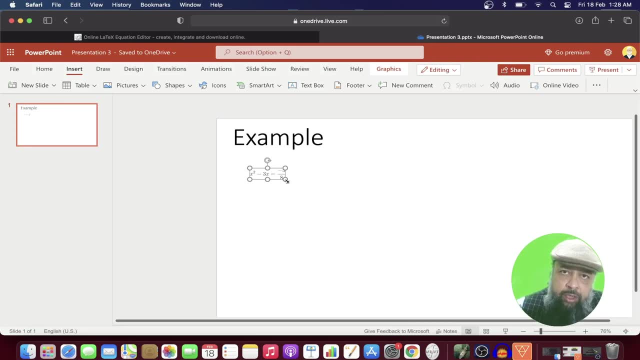 the right hand side, PowerPoint is giving me some suggestions. If I don't want to use these suggestions, I can close this and this is my image, And if I hover over this corner, lower right corner, I can resize this. as you can see that, as I am increasing the size of the 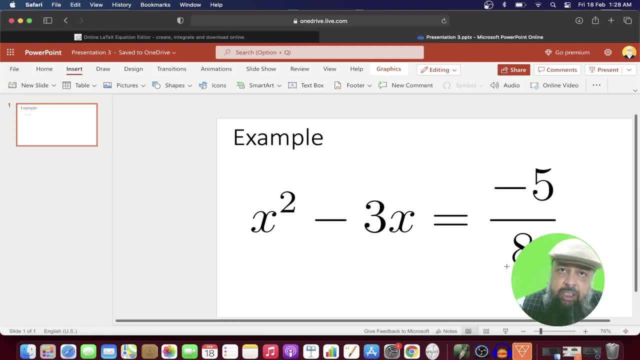 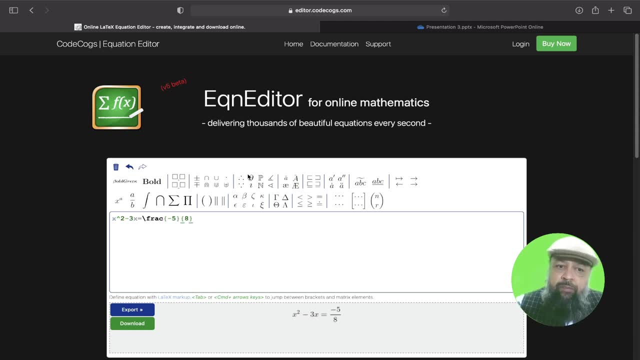 image. the sharpness of this math equation stays the same, which is awesome because this is a vector file in your math expressions. you will have some fractions, you will have some symbols, subscript, superscript. So I have already explained how to use superscript for subscript. Let me give you 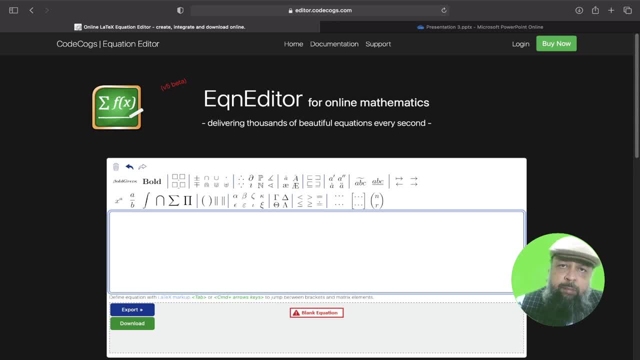 another example in which I have to type x subscript one plus x subscript two. just an example. So for this I type x underscore. one underscore is for subscript plus x. underscore two and so on is equal to, let's say, minus five. So this is how. 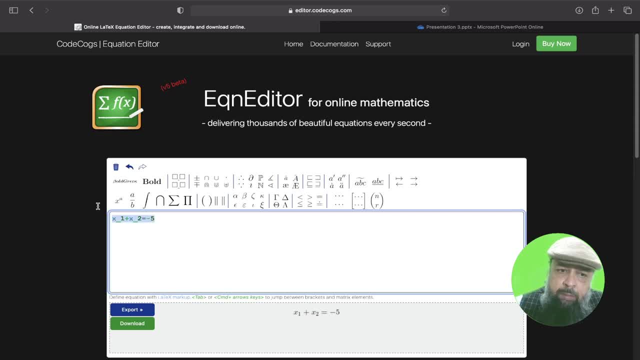 you can type subscript. So similarly for matrices, if I click on that, I can choose how many rows and columns my matrix has. And as you can see that there are three rows and three columns And if I click my mouse, a matrix environment will. 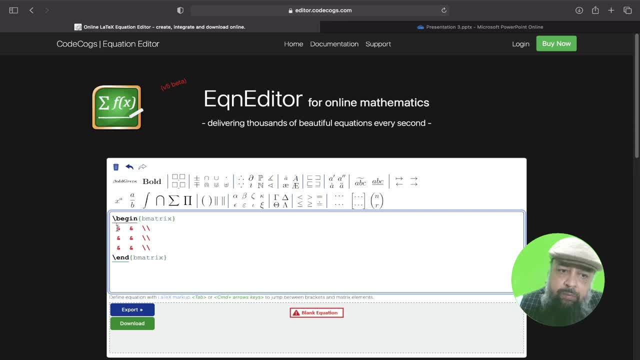 be placed in this editor And I simply have to type the elements of this matrix before this M percent sign. So let's say one is the first element, then two and then three, And these two backslashes means new line. let's say minus, four, minus. 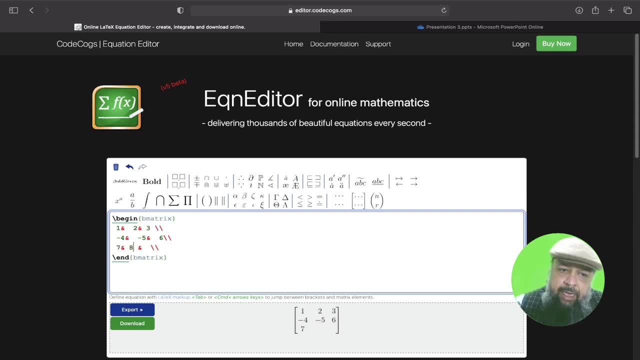 five, six, seven, eight, nine, And this is my matrix, And now I can simply download and insert into my presentation, as I explained earlier. So this is how you can type matrices. So let me show you an example For integral. if I hover over this integral, as you can see, 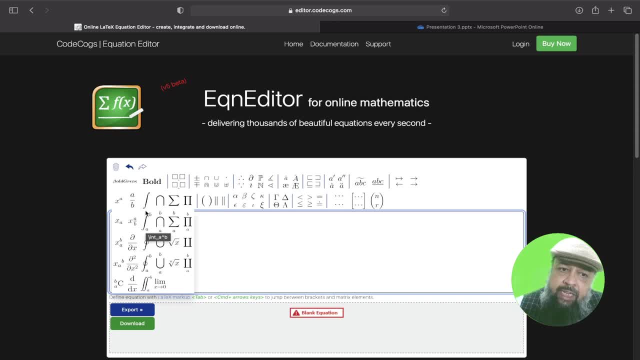 that there are many types of integrals available. For example, this is a simple integral, no upper or lower limits. you simply type backslash int for integral with limits. you type in this manner: backslash int for integral. underscore a means. 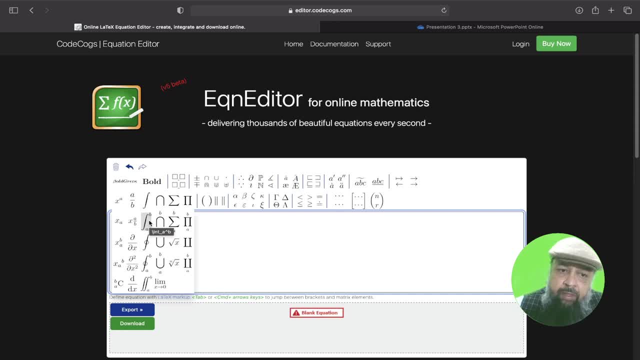 lower limit, just like subscript. And hat B means upper limit is B. So in this way you can type integral, for example, if you want the lower limit to be zero and upper limit to be infinite. So after this hat, you type I n, f, t, y, which is the symbol for 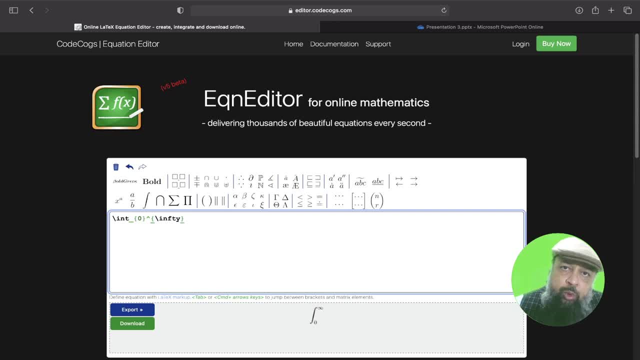 infinity, And then after that you have to type some expression. to do that, you put curly brackets, And when you type left side curly bracket, the right will be automatically inserted. Now you can type any thing, for example minus sine x and these: 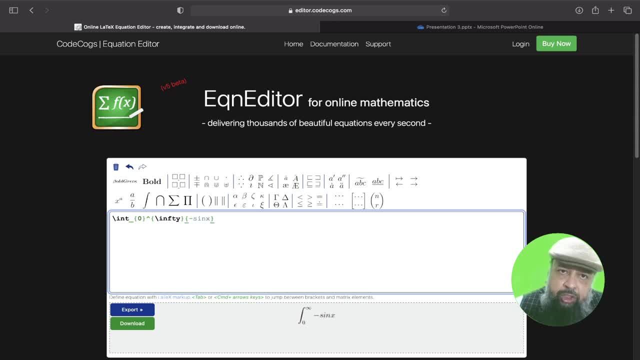 curly brackets will not appear in the expression. And if you want to make them appear, then then you put backslash and then curly brackets around this whole expression and now they will appear. So these are little things. you have to understand how to put the brackets, or to put subscript, superscript And 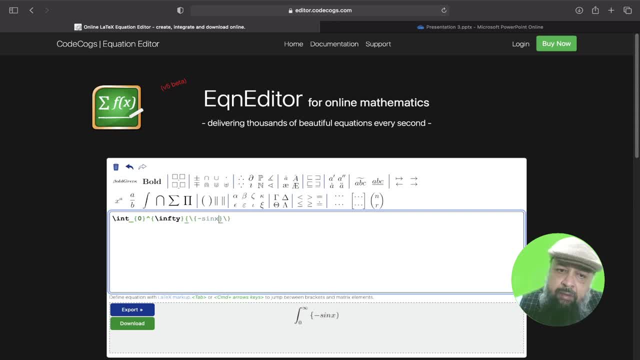 these are very easy. So if you want to put, for example, parentheses, you can simply put it like this: So one pair of curly brackets is used as a bracket, But if you want to show the bracket, you have to use backslash and then the curly bracket. So let me show you. 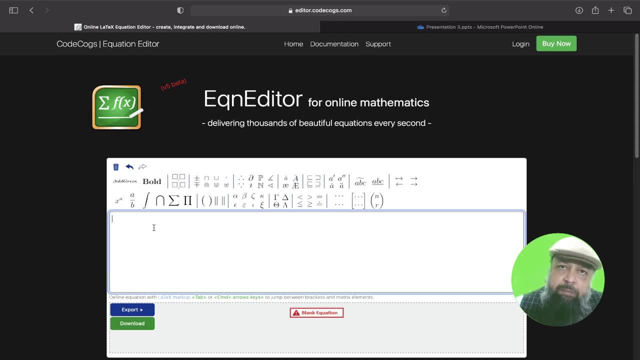 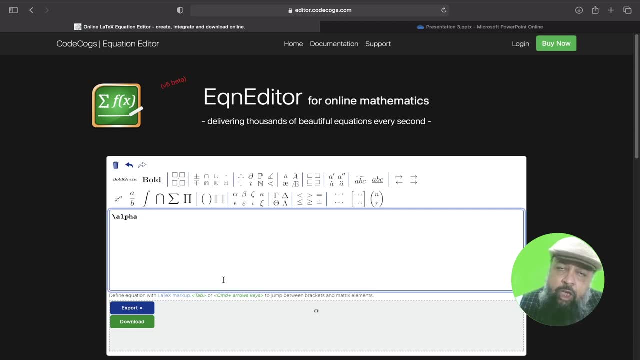 another example. For example, I want to put alpha plus beta plus gamma equals zero. So I click on alpha, alpha will be placed. then I type plus on my keyboard, then I click on beta and backslash. beta is the later command to print beta. And then I put plus sign and gamma is.